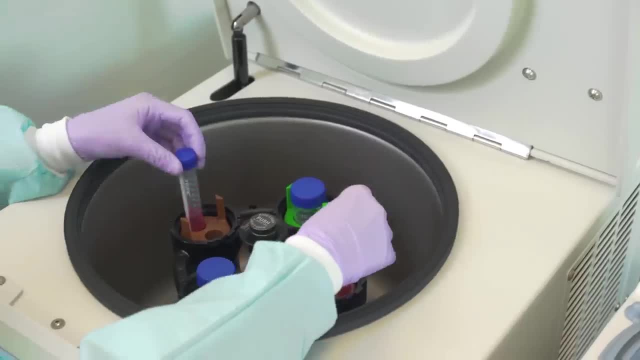 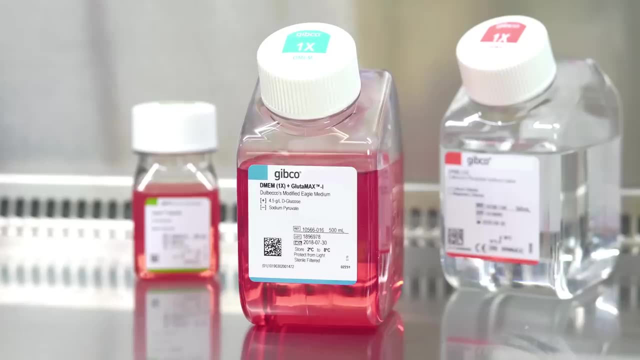 hood, an incubator, a water bath, a centrifuge, a refrigerator-freezer, a hemocytometer and a microscope. You'll also need cell culture, flasks, medium and other reagents, pipettes and waste containers. The hood provides a sterile environment to work with your cells. 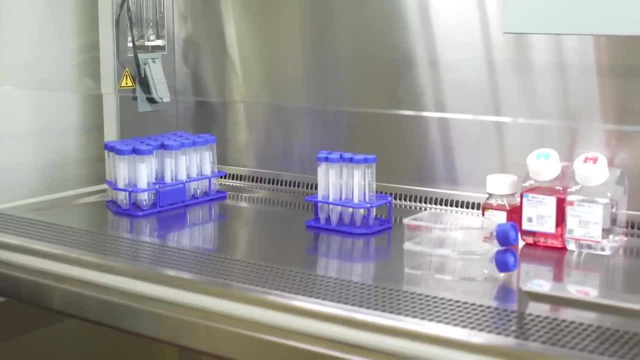 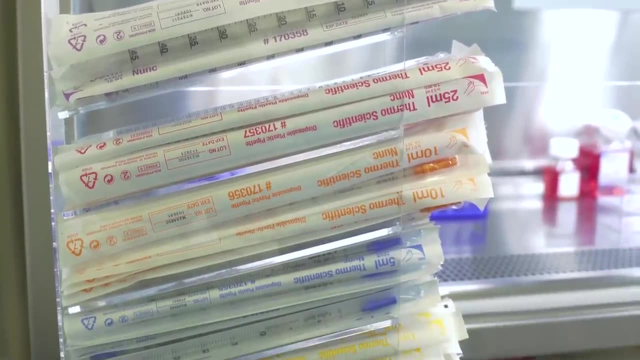 without fear of contamination. Always open your cell culture dishes and reagent bottles in a sterile environment. Outside the cell culture hood keep a stack of disposable pipettes nearby. Pipettes are placed in the hood during use and only opened inside the sterile field. 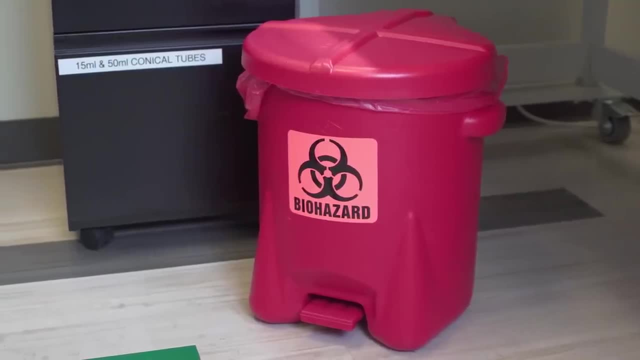 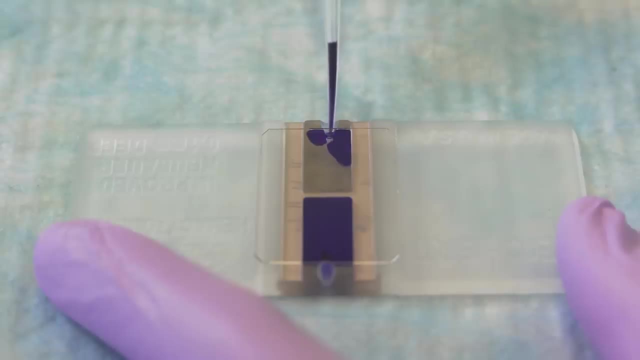 Have the trash, biohazard bin and sharps container close by A cell counting machine such as the Countess gives you quick, accurate counts needed during culturing, Or you can count cells manually with a hemocytometer. You may also wish to have the centrifuge located. 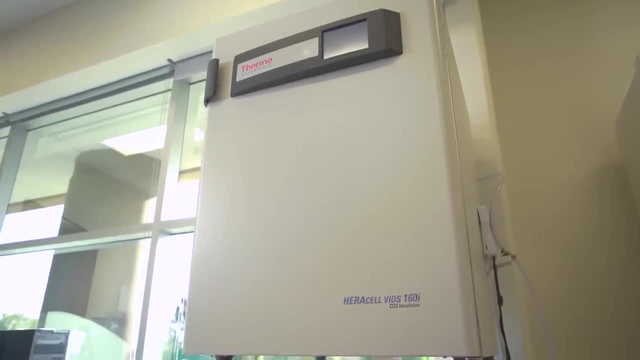 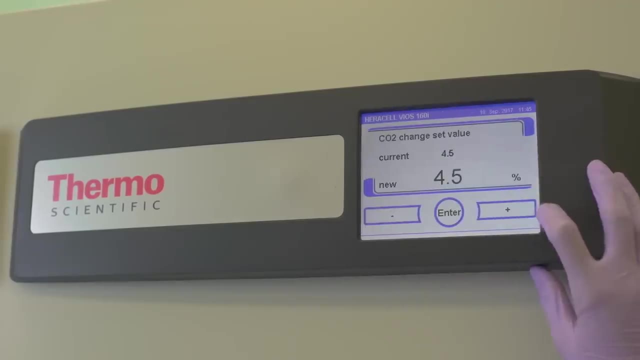 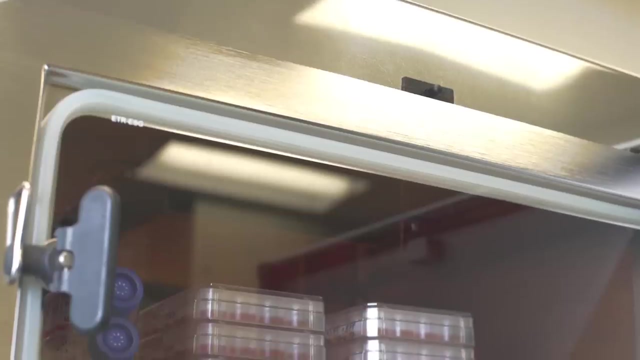 in the cell culture facility. Incubators provide the appropriate environment for cell growth. Carbon dioxide and temperature settings are also required. Cell type and medium selection. Mammalian cells are cultured at 37 degrees Celsius in the presence of 5 to 7 percent carbon dioxide with high humidity Inside the incubator. 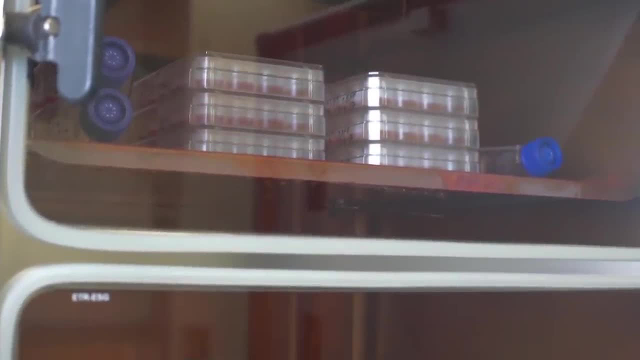 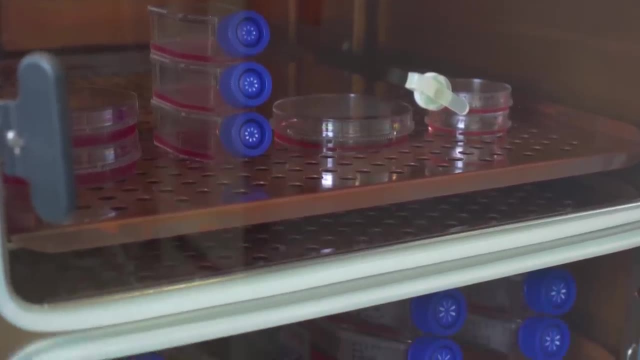 keep your cell culture flasks evenly spaced and avoid crowding to ensure that the air inside the incubator moves freely. This helps to maintain temperature, humidity and proper gas exchange. Don't make very tall stacks of plates. They may fall over and lower ones. 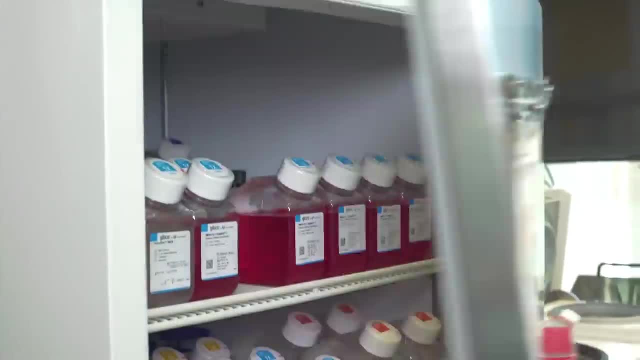 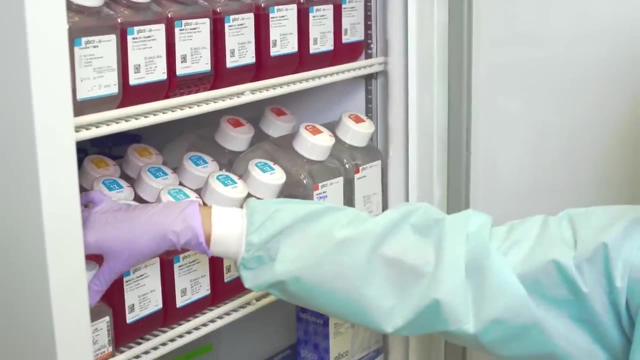 may not get the appropriate gas exchange. Store all media and reagents in a storage bag. Some components are known to degrade when left at room temperature or exposed to light for extended times. If the medium will be stored in a glass front refrigerator or a. 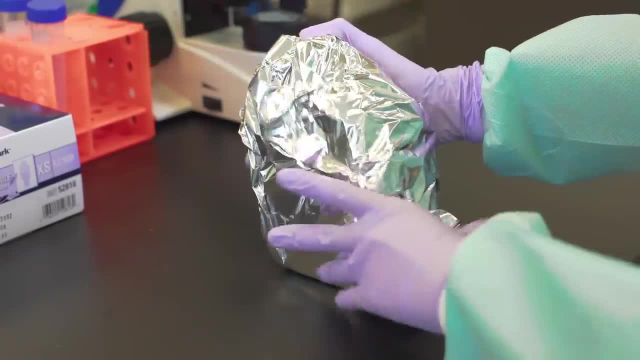 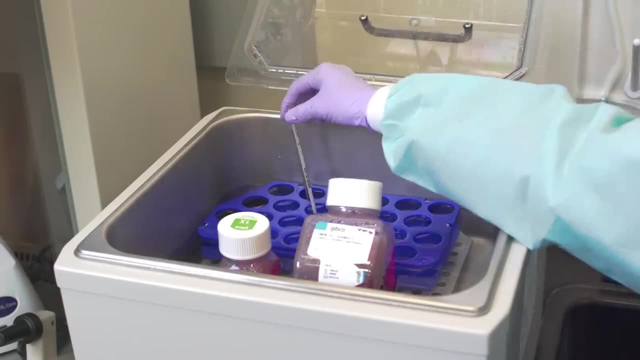 cold room, wrap the bottles in tinfoil or store them inside a box. Some labs warm their reagents to 37 degrees Celsius before use. Warming reagents should take 10 to 20 minutes, depending upon the size of bottles you are using. Others choose to use reagents warmed. 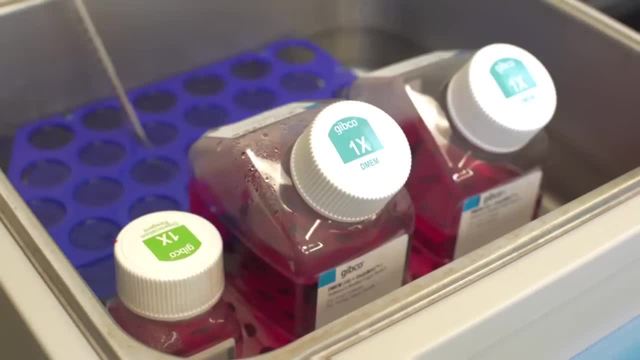 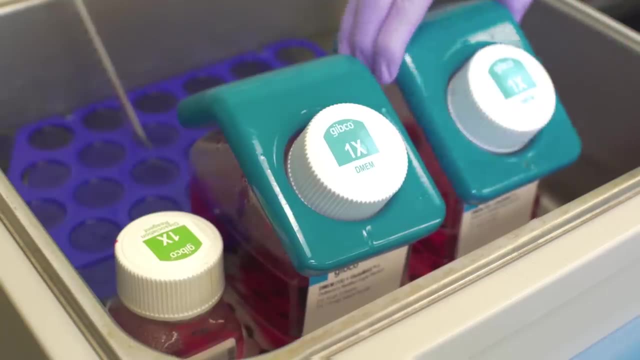 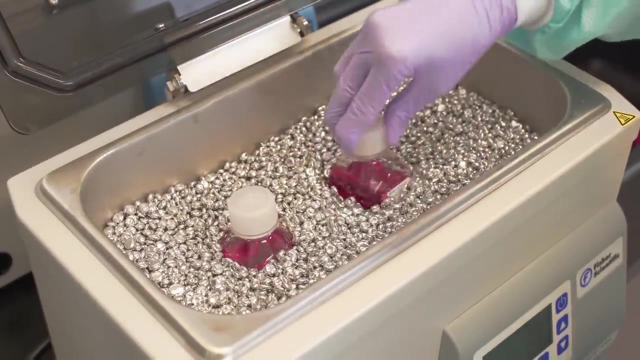 to room temperature. If you use a water bath, make sure to keep bottles upright with necks out of the water. Specially designed bottle weights are available for use with the Gibco bottle. Alternatively, metallic bath beads can be used instead of water. Bath beads are a cleaner, greener alternative.